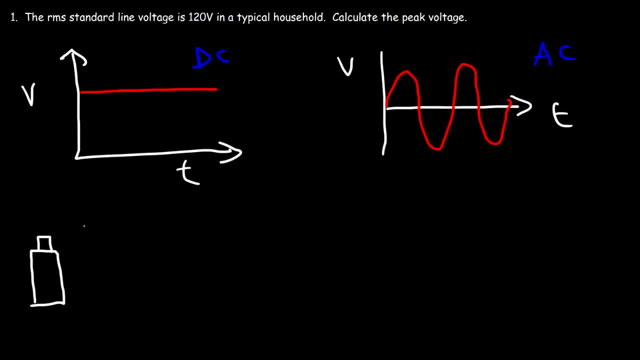 Now a DC current is available if you use a device like a battery, If you connect the battery across a resistor or even a light bulb, current flows in one direction. The conventional current flows from the positive terminal of the battery towards the negative terminal of the battery. Now let's say, if you connect a resistor across a 120 volt source, 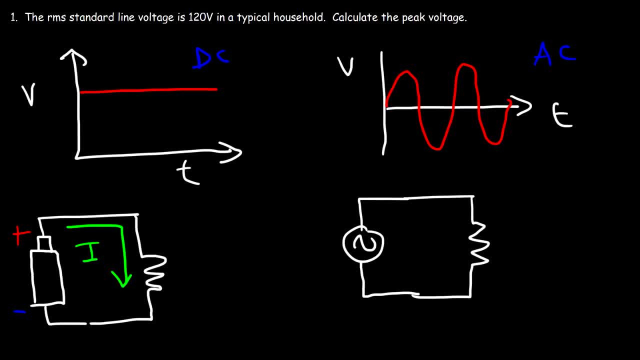 current flows from the positive terminal of the battery to the negative terminal of the battery. Now, in this case, the current constantly reverses direction. In one instance it's traveling in this direction and then in another instance, it's traveling in the 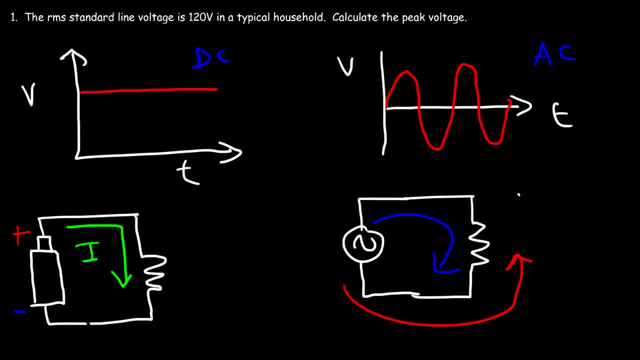 opposite direction, And so it oscillates 60 times per second, And so the frequency is 60 hertz. It constantly reverses 60 times in one single second. So that's the difference between DC current and AC current. 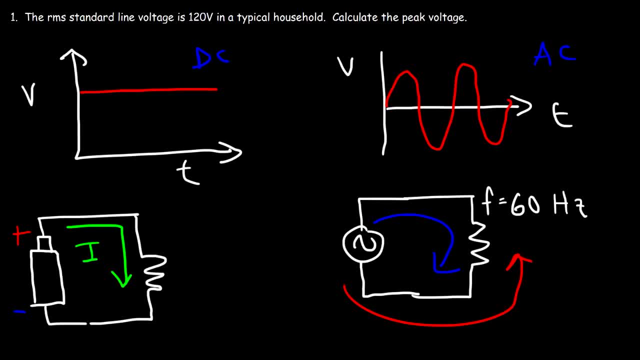 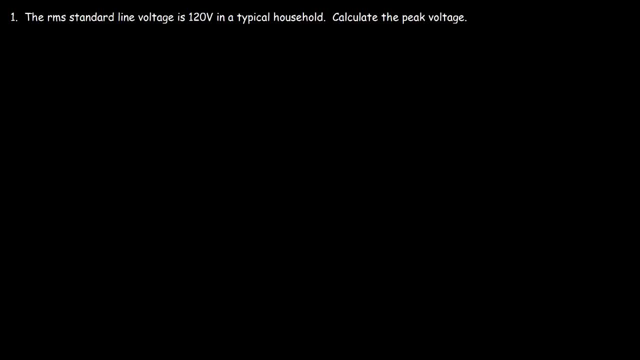 Now let's go back to this problem. The RMS standard line voltage is 120 volts in a typical household. Calculate the peak voltage. The peak voltage is equal to the square root of 2 multiplied by the RMS voltage. So the RMS voltage is 120 volts and if we multiply that, 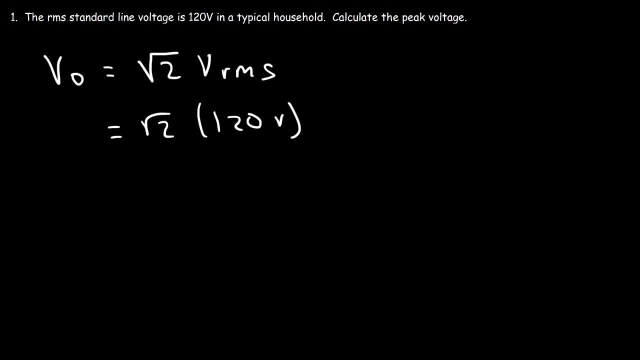 by the square root of 2, this is going to equal 169.7 volts. You can approximate it and say it's about 170 volts. So that's the peak voltage found in a typical household line. Number 2, consider the sinusoidal function. 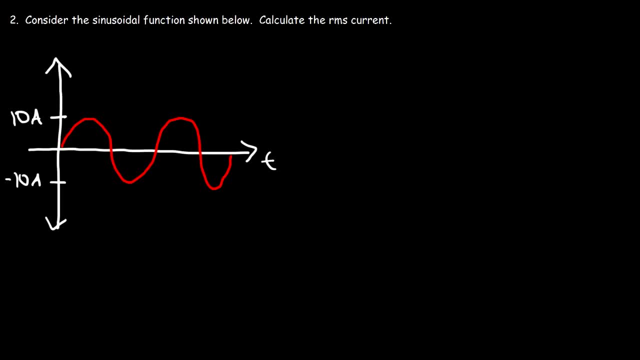 shown below. Calculate the RMS current that's flowing in the circuit. If this graph represents the current flowing from one of the strategies, that would be 2.1 volts. If this graph represents the current flowing from one of the materials, that's 0.020 volts. And if we multiply that we will says this equals 1.007.8 volts. So this is 160 volts And lets say that 60 volts, But if this graph represents the RMS current and if we estimate that it reaches abrebeult, 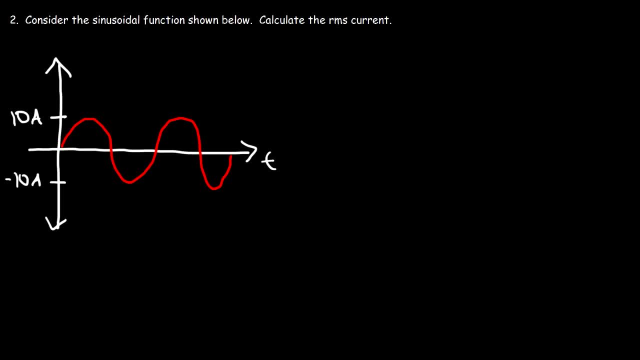 which is always based on those. why's close? and in between, diethyl and to the favourite'ves, the difference in eachics of voltage flowing in a circuit at any given instant of time. so what is the peak current? the peak current is the maximum current. the maximum current is 10 amps. 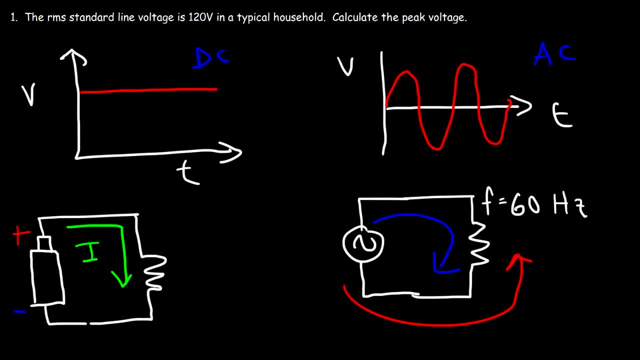 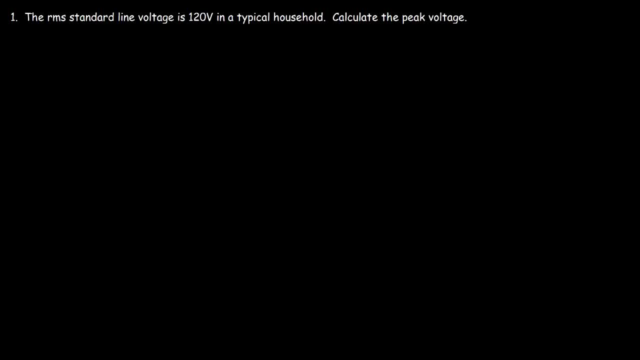 Direct current and alternating current. Now let's go back to this problem. The RMS standard line voltage is 120 volts in a typical household. Calculate the peak voltage. The peak voltage is equal to the square root of 2 multiplied by the RMS voltage. So the RMS voltage is 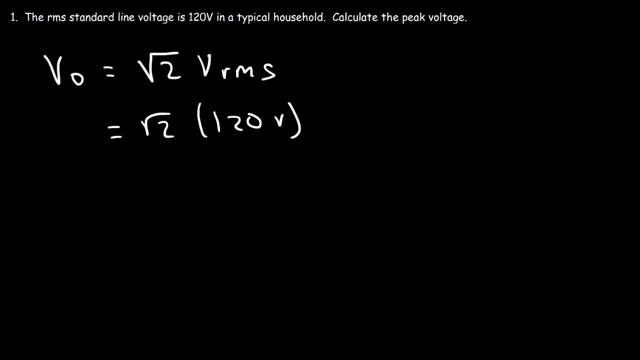 120 volts And if we multiply that by the square root of 2, we get the RMS voltage. The RMS voltage is equal to the square root of 1. multiplied by the RMS voltage, This is going to equal 169.7 volts. You can approximate and say it's about 170 volts, So that's. 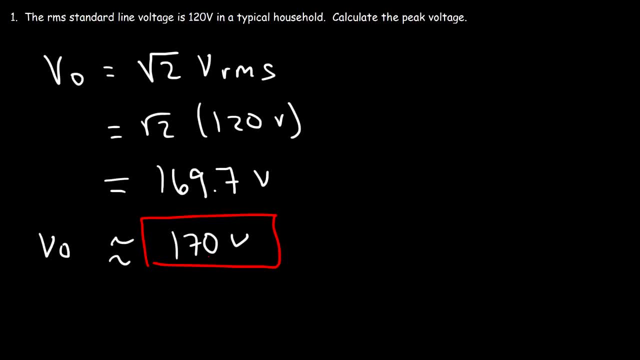 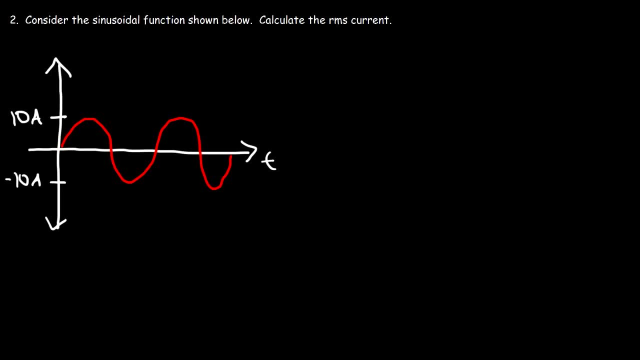 the peak voltage found in a typical household line. Number two: consider the sinusoidal function shown below: Calculate the RMS current that's flowing in the circuit. If this graph represents the current flowing in the circuit at any given instant of time, you can calculate the RMS current that's flowing in the circuit. 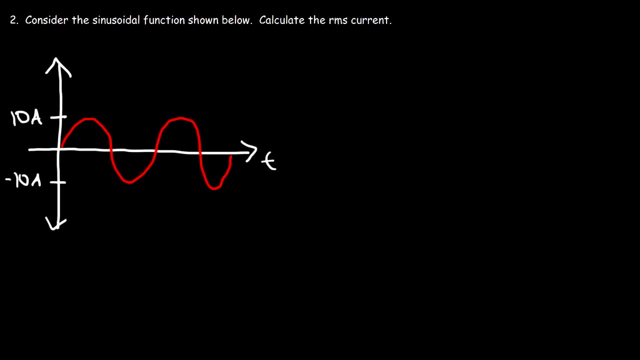 time. So what is the peak current? The peak current is the maximum current. The maximum current is 10 amps. So if we want to calculate the RMS current, it's going to be the peak current divided by the square root of 2.. So it's 10 amps over the square root of 2.. And so this is going to equal 7.07 amps. So that's how you can calculate the RMS current from the peak current Number 3.. A 200 watt laptop is connected to a 240 volt AC line. Calculate the RMS current flowing from the outlet. So we have the average power. 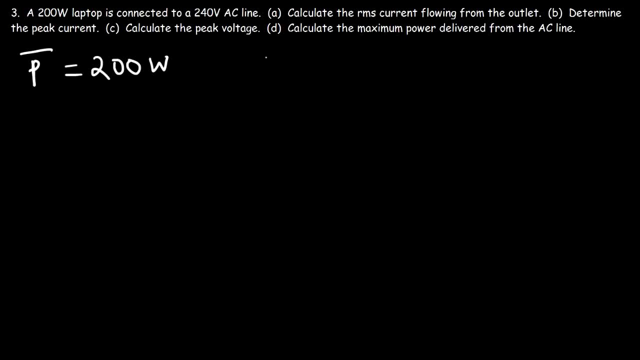 That's consumed by the laptop, It's 200 watts And the line voltage that represents the RMS voltage, the root mean square voltage, And so that's 240.. So in part A, our goal is to calculate the RMS current. The average power is simply equal to the RMS voltage times. 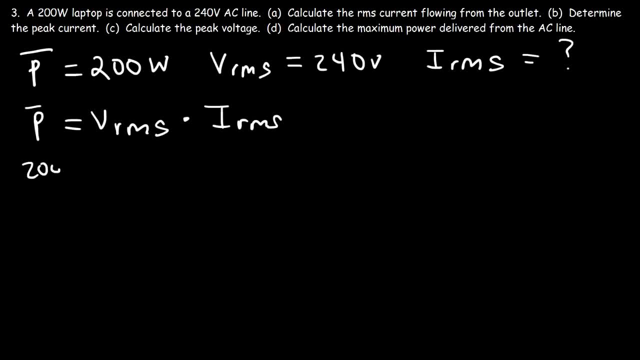 the RMS current, And so this is 200 watts. That's going to equal 240 times the missing current value. So the RMS current is going to be 200 watts divided by 240 volts, And so that's equal to 0.8333 amps. Now let's calculate the peak current. The peak current is the square root. 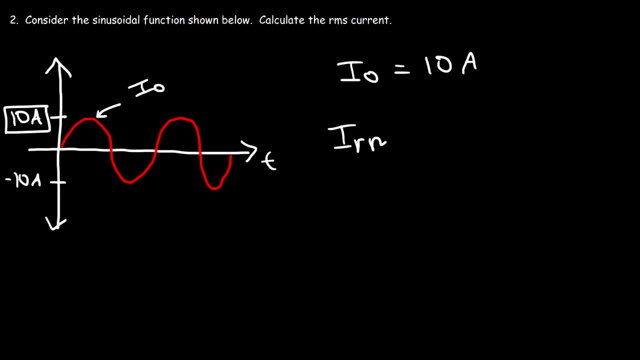 so if we want to calculate the RMS current, it's going to be the peak current divided by the square root of 2, so it's 10 amps over the square root of 2, and so this is going to equal seven point zero seven amps. so that's how you. 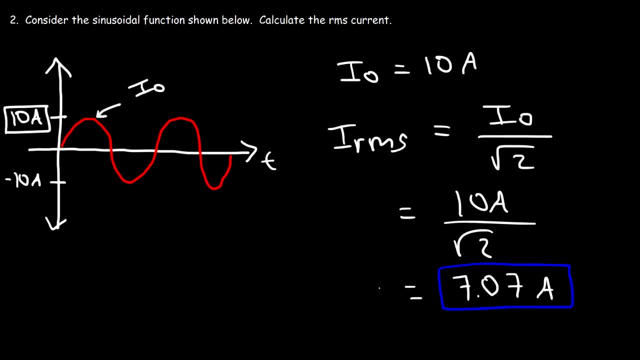 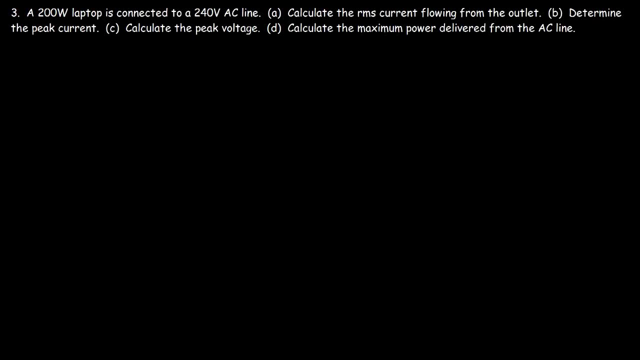 can calculate the RMS current from the peak current. number three: a 200 watt laptop is connected to a 240 volt AC line. calculate the RMS current flowing from the outlet. so we have the average power that's consumed by the laptop. it's 200 watts and 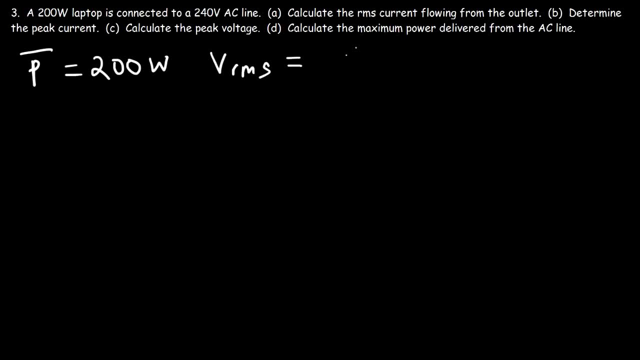 the line voltage that represents the RMS voltage to root mean square voltage, and so that's 240. so in part a our goal is to calculate the RMS current. the average power is simply equal to the RMS voltage times the RMS current, and so this is 200. 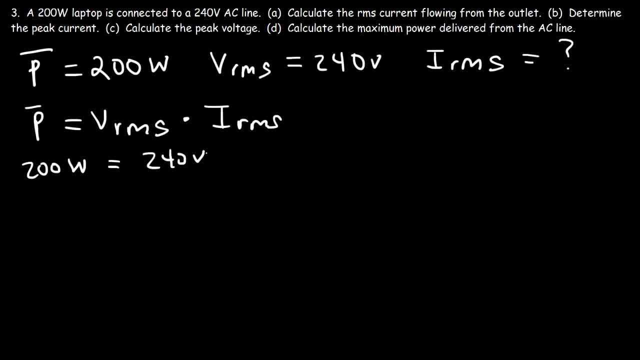 watts, that's going to equal 240 times the missing current value. so the RMS current is going to be 200 watts divided by 240 volts, and so that's equal to 0.8 333 amps. now let's calculate the peak current. the peak current is the square. 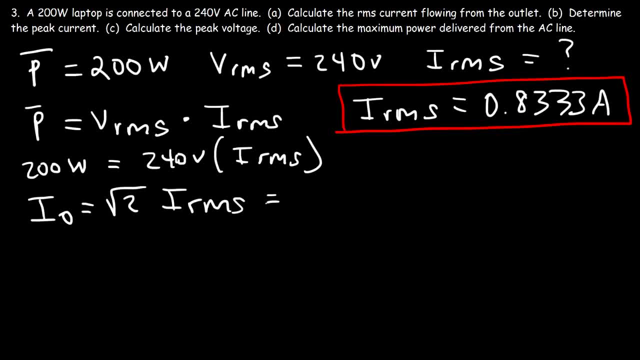 root of 2 times the RMS current, and so it's going to be the square root of 2 times point 8333, and so this is equal to one point 1785 amps. now part c, the peak voltage. the peak voltage is going to be the square root of 2 times. 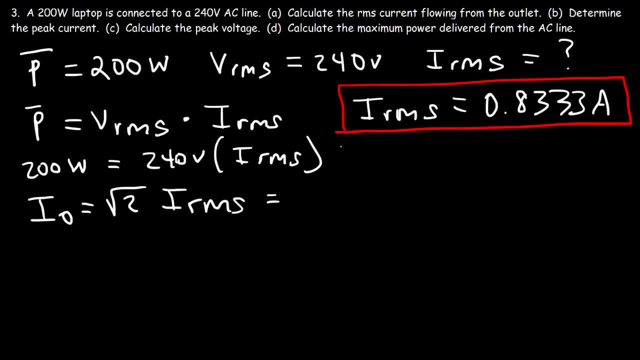 of 2 times the RMS current, And so it's going to be the square root of 2 times the RMS current. Now you get a lot of the RMS current. The RMS current is 0.8333.. The RMS current is 0.8333.. The unit current is 0.8333.. And so this is equal to 1.1785 amps. Now, part C: Calculate the peak voltage. The peak voltage's going to be the square root of 2 times the RMS current. 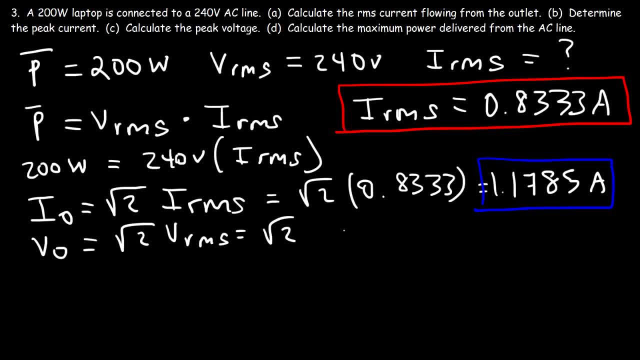 Now this is going to be 1.1785 Amps. Now I'm going to take the RMS current and choose the RMS current Number 3.. A 250 watt laptop VRMS, so that's the square root of 2 times 240 volts, and so that's going to. 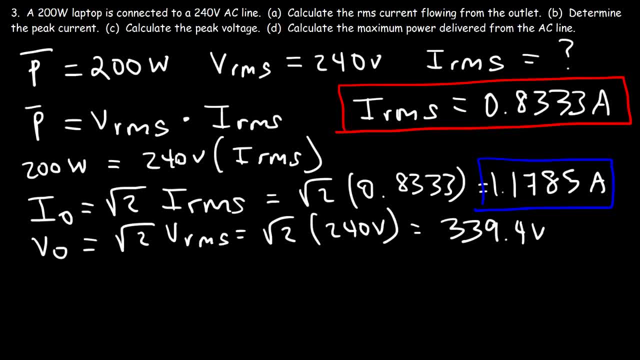 be 339.4 volts. now let's move on to Part D. calculate the maximum power delivered from the AC line. the maximum power is equal to the peak voltage times the peak current. so that's going to be the peak voltage is 339.4 x 1.1785, and so the 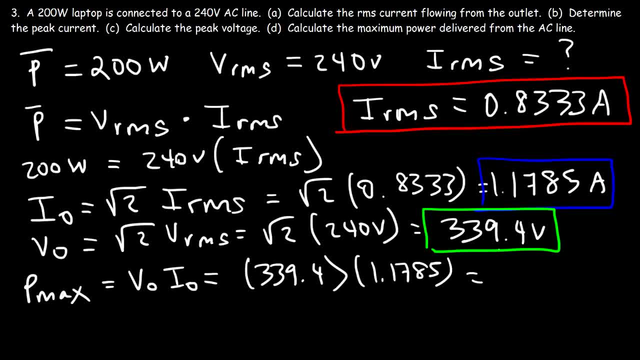 maximum power is 399.98, which you could say it's about 400 watts. now it's important to understand that the maximum power is twice the value of the average power, which means the average power is one-half of the maximum power. so in this case we could have done two times 200 watts and that would have. 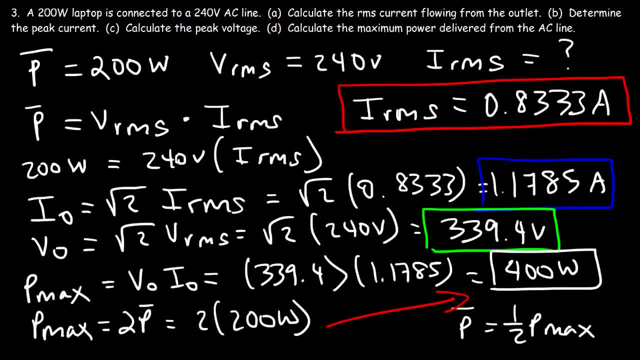 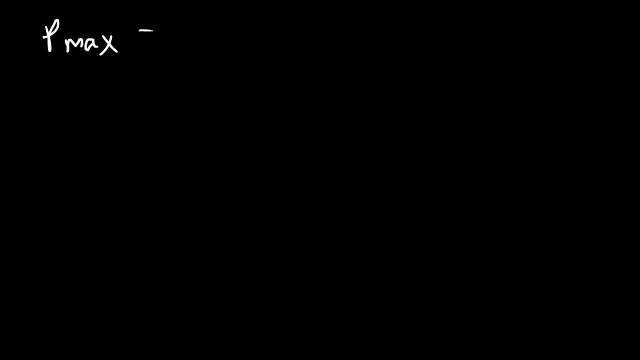 given us 400 watch, which is the maximum power. so let's talk about some formulas they need to know. they need to know that the maximum power is simply the peak voltage times the peak current, and the average power is the RMS voltage times the RMS current. now let's say, if you want to get the maximum power in terms 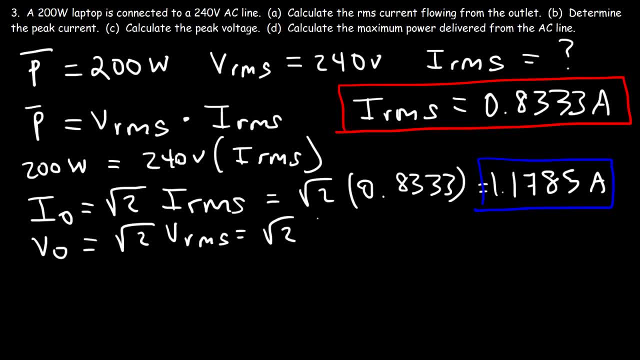 V RMS. so that's the square root of 2 times 240 volts, and so that's going to be 339 point 4 volts. now let's move on to Part D. calculate the maximum power delivered from the AC line. the maximum power is equal to the peak voltage times. 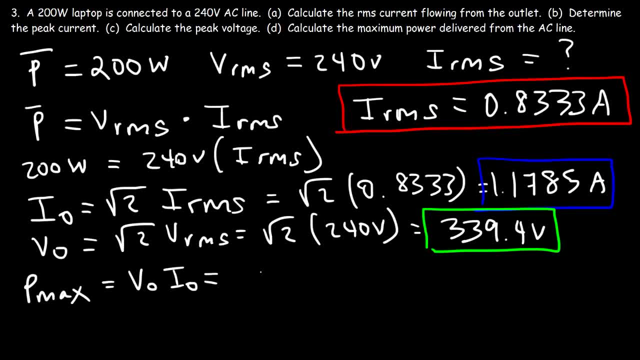 the peak current. so that's going to be the peak voltage is 339 point 4 multiplied by one point one, seven, eight, five, and so the maximum power is three hundred ninety nine point nine eight, which you could say it's about 400 watts. now it's important to understand that the 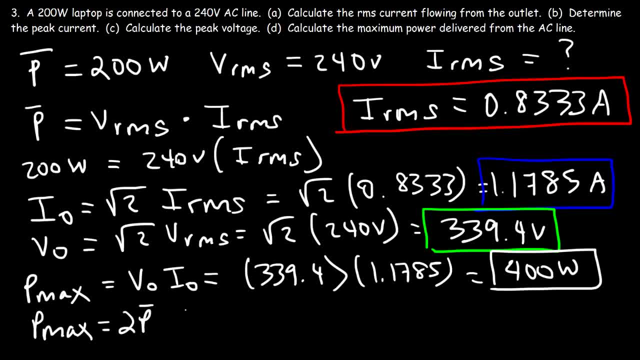 maximum power is twice the value of the average power, which means the average power is one half of the maximum power. so in this case we could have done two times 200 watts, and that would have given us 400 watch, which is the maximum power. so let's talk about some formulas that you need to know, so you need to. 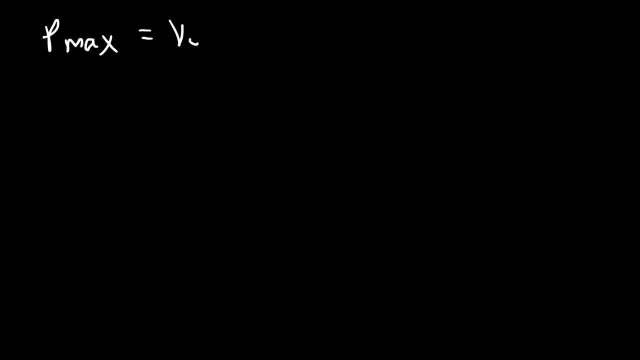 know that the maximum power is simply the peak voltage times the peak current, and the average power is the RMS voltage times the RMS current. now let's say: if you want to get the maximum power in terms of these values? so let's focus on this equation now. we 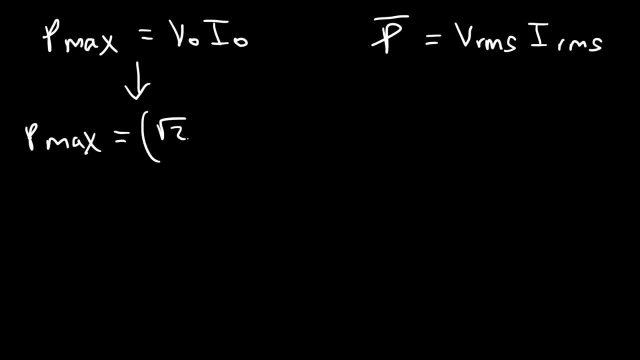 know that the peak voltage is the square root of 2 times the RMS voltage and the current is a square root of two times the RMS voltage. current now the square root of 2 times the square root of 2, that's equal to the square root of 4, which is 2, so the maximum power it's 2 times the RMS. 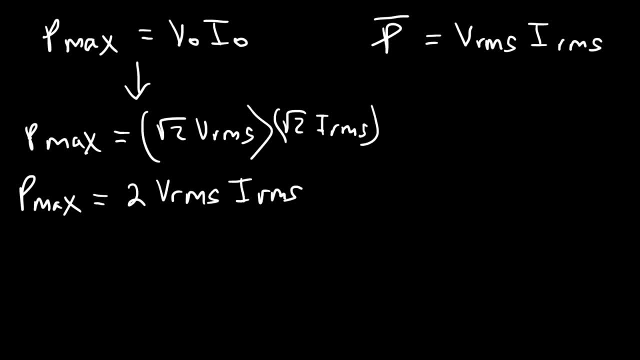 voltage times the RMS current. so those are the two main ways to calculate the maximum power. and, as we said before, this is equal to the average power. so the maximum power is twice the value of the average power. now let's focus on this equation. now we can get the average power in terms of these values. so VRMS. 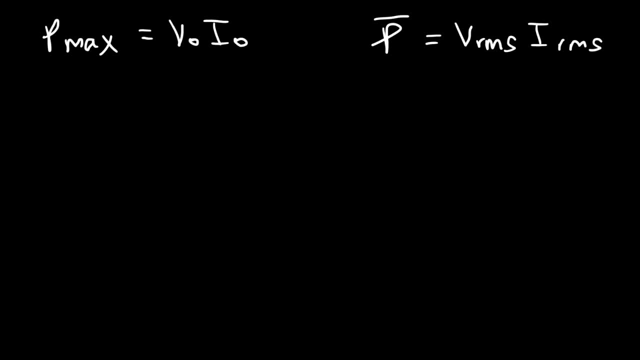 of these values. so let's focus on this equation now. we know that the peak voltage is the square root of 2 times the RMS voltage, and the peak current is the square root of 2 times the RMS current. now the The square root of 2 times the square root of 2, that's equal to the square root of 4, which is 2.. 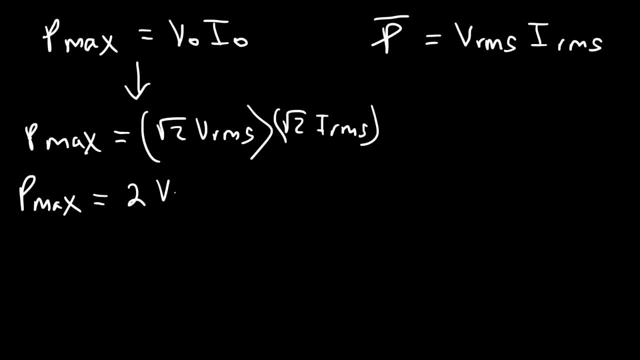 So the maximum power is 2 times the RMS voltage, times the RMS current. So those are the two main ways to calculate the maximum power And, as we said before, this is equal to the average power. So the maximum power is twice the value of the average power. 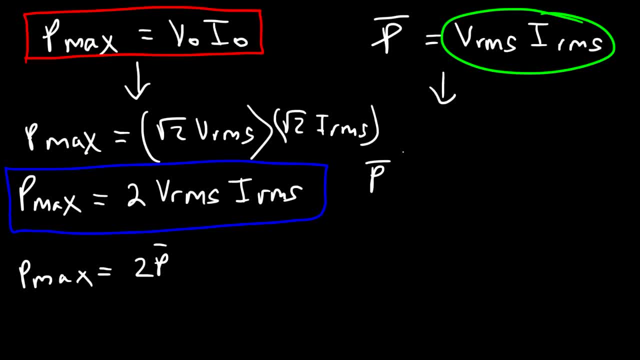 Now let's focus on this equation. Now we can get the average power in terms of these values. So VRMS is equal to the peak voltage divided by the square root of 2.. And the RMS current is equal to the peak current divided by the square root of 2.. 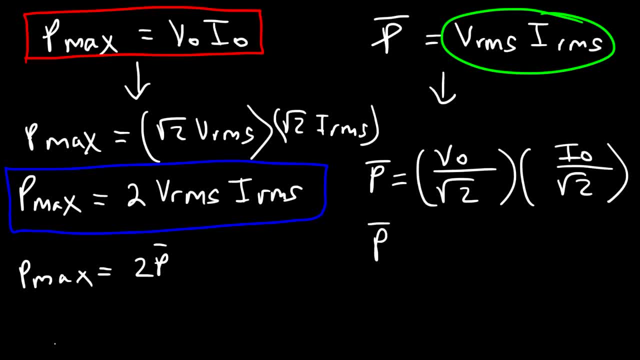 So these two together will give us a 2 on the bottom. So therefore we can say that the average power is simply 1. 1.5 of the peak voltage times the peak current, And the peak voltage times the peak current represents the maximum power. 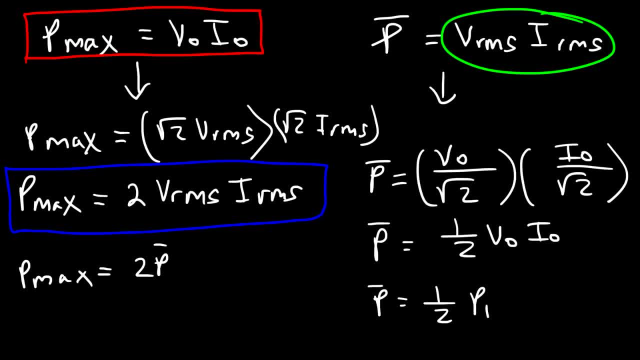 So that's why we can say that the average power is 1.5 of the maximum power. So make sure you know these formulas, Because you can use it in different ways. Number 4. Now, this is going to be the last problem of this video. 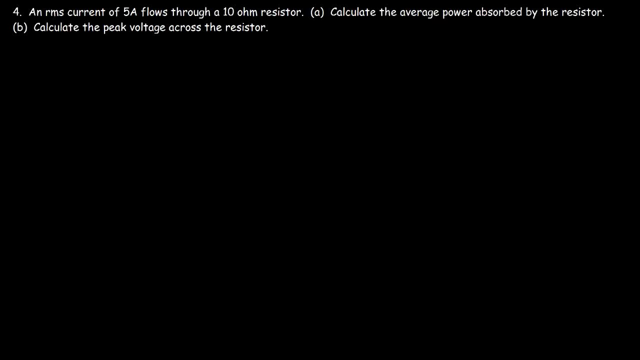 An RMS current of 5 amps flows through a 10 ohm resistor. Calculate the average power absorbed by the resistor. So if we draw a circuit, Let's say this is the AC power source And here we have a 10 ohm resistor. 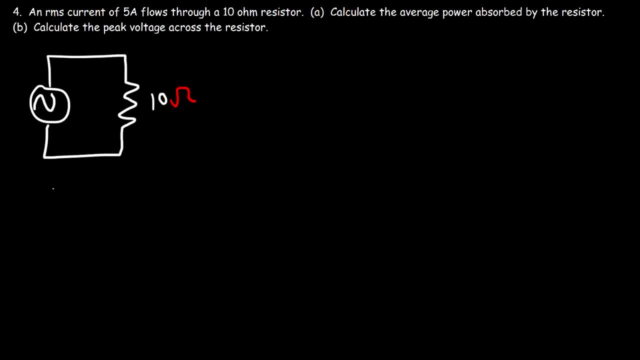 So the current that's oscillating in this circuit It's really going in both directions, So keep that in mind. The current is 5. And the resistance is 3.. So the voltage is 2. And the resistance is 3.. 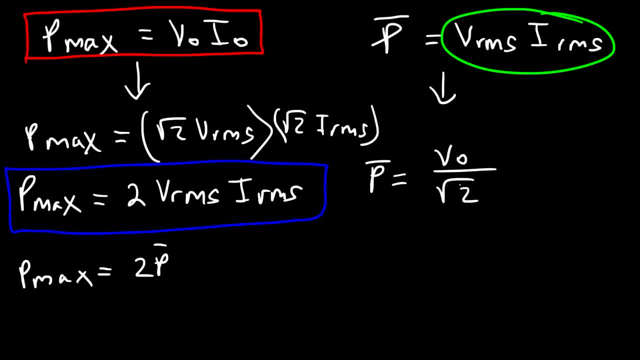 is equal to the peak voltage divided by the square root of 2, and the RMS current is equal to the peak current divided by the square root of 2, so these two together will give us a 2 on the bottom. so therefore we can say that the 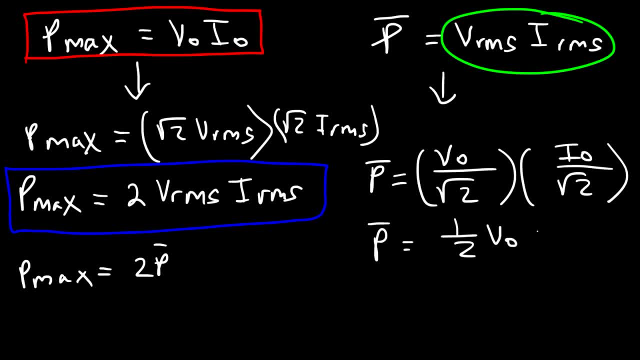 average power is simply 1 half of the peak voltage times the peak current, and the peak voltage times the peak current represents the maximum power. so that's we can say that the average power is 1 half of the maximum power. so make sure you know these. 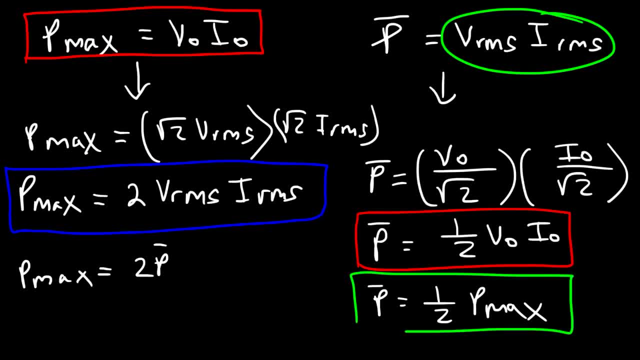 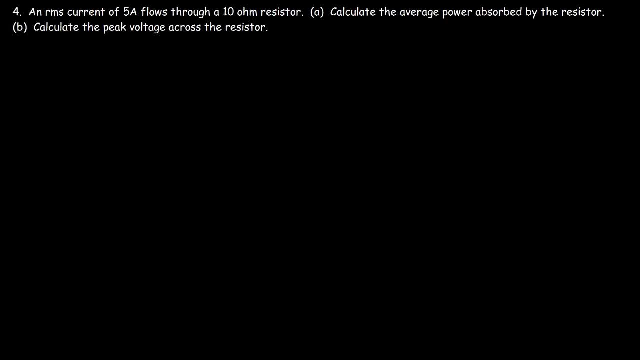 formulas because you can use it in different ways. number four: now this is going to be the last problem of this video. an RMS current of 5 amps flows through a 10 ohm resistor. calculate the average power absorbed by the resistor. so if we draw a circuit, let's say this is the AC power source. 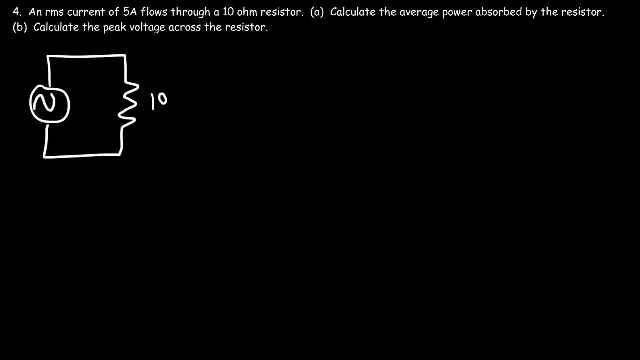 and here we have a 10 ohm resistor. so the current that's oscillating in this circuit it's really going in both directions, so keep that in mind. the current is 5 amps, so how can we calculate the average power? the average power is the RMS. 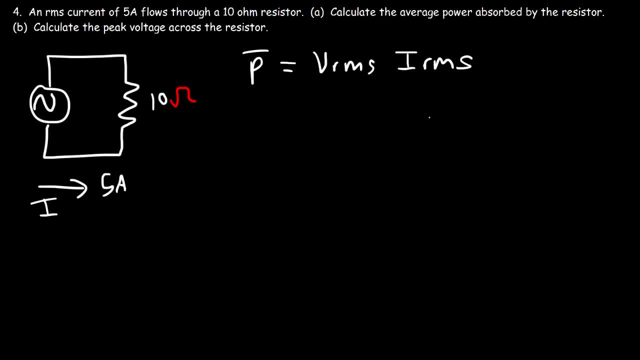 voltage times. the RMS current and based on Ohm's law V is equal to IR. so the RMS voltage is equal to the RMS current times of resistance. so what I'm going to do is replace the RMS voltage with the RMS current times of resistance. so if we 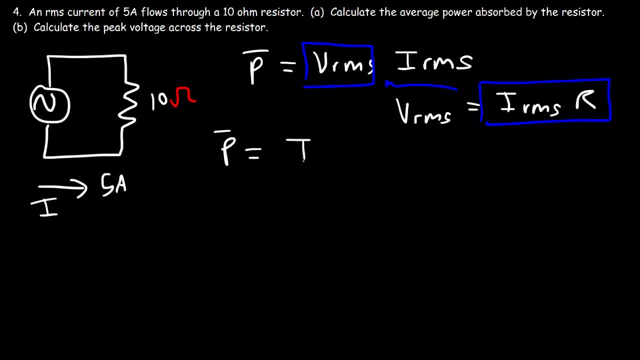 plug that in this is going to be equal to the current times, the resistance times another current value. so the average power is the square of the RMS current multiplied by the resistance. you can also say that it's 1 half of the square of the peak current times, the resistance. but we're 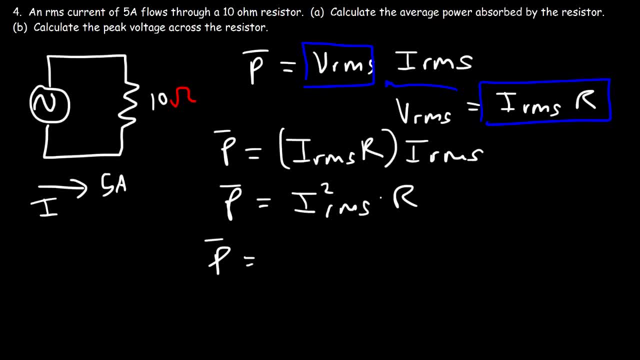 not going to use that equation in this example, since we already have the RMS current. so the RMS current is 5 amps and we need to square it and the resistance is 10 ohms. 5 squared is 25, and 25 times 10 is 250. so the average power absorbed.